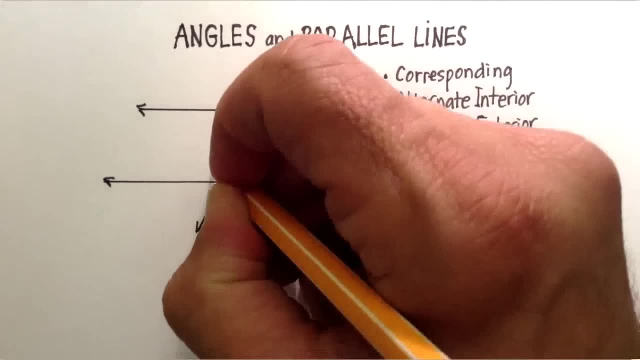 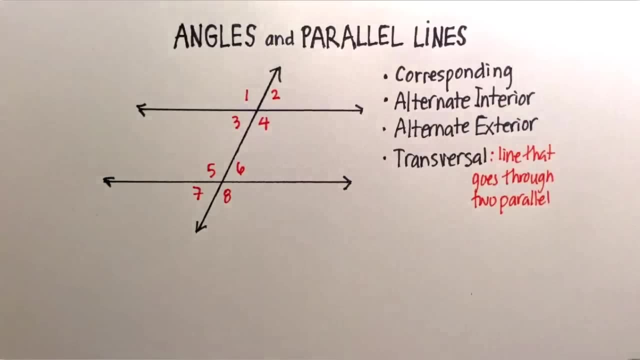 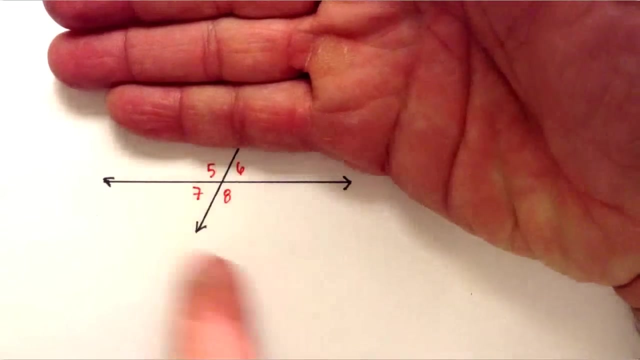 One, two, three, four, five, six, seven and eight. Now, what you'll notice here is that when the transversal cuts through one parallel line, you have four angles, don't you? Two on the top, two on the bottom, 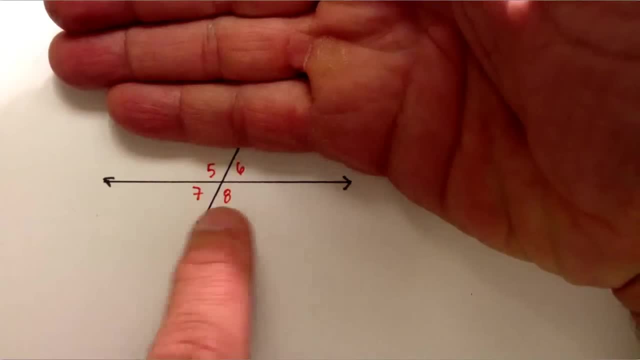 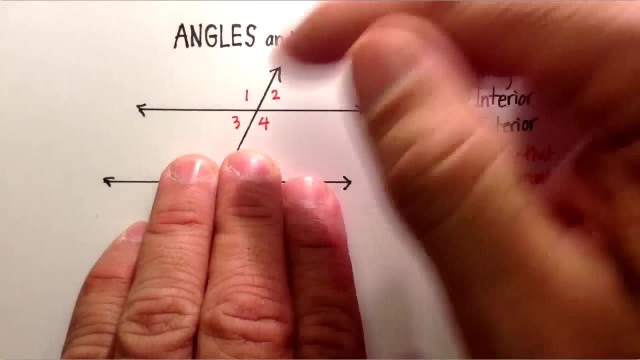 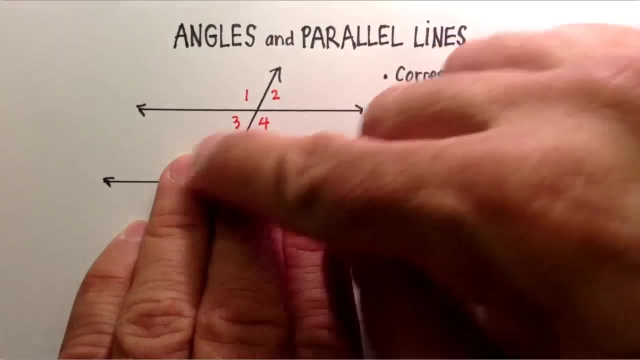 We'll go like upper left, upper right, lower right, lower left. okay, But it also forms that same grouping on the top part, on the other parallel line, right, You have an upper left, an upper right, a lower right. 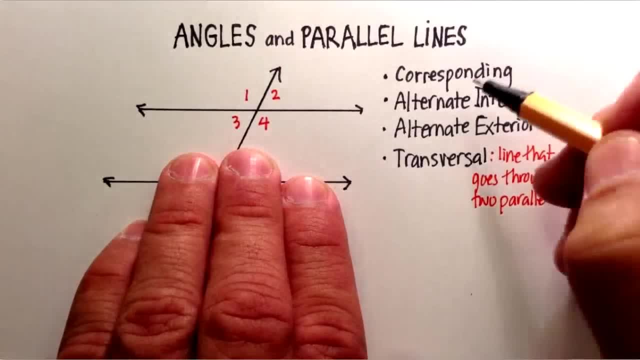 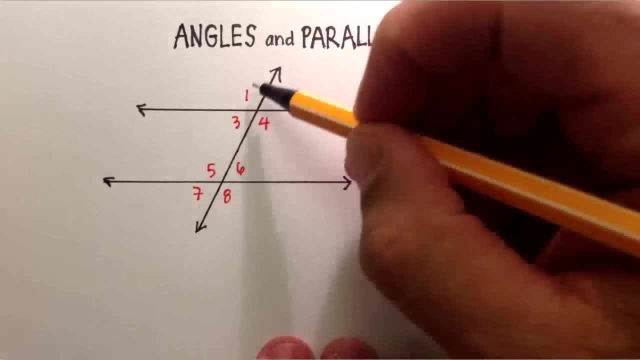 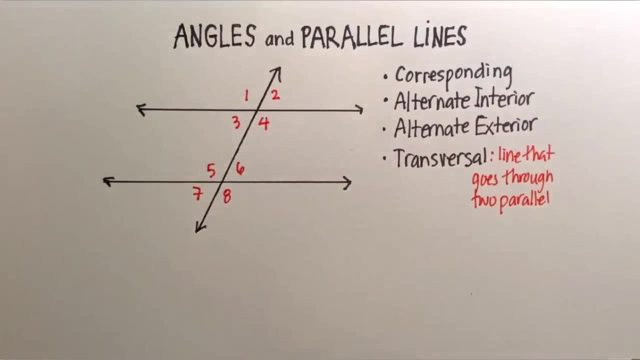 and a lower left. So now we're going to talk about what's called corresponding angles. Corresponding angles are the angles that are formed that are in the same spot in each of the groupings. Okay, so, for example, angle one and angle five would be corresponding angles. 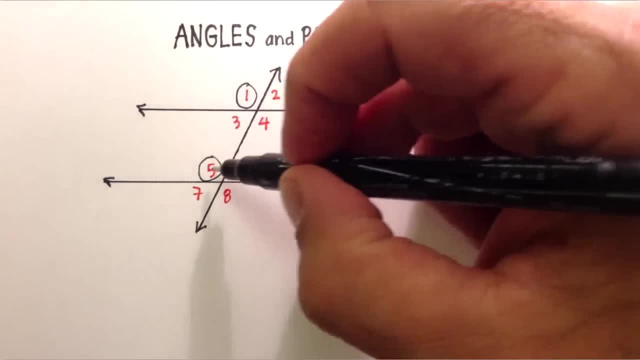 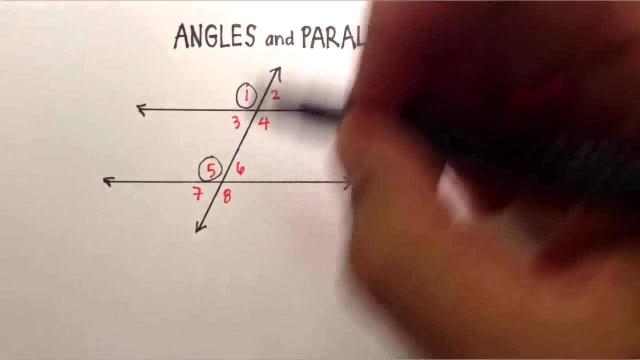 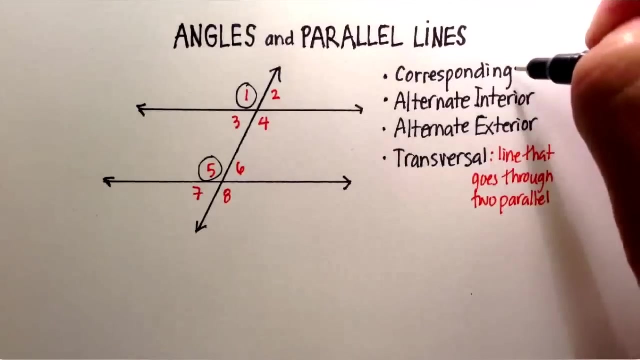 because they're both in the upper left-hand side of their grouping. Okay, So the top grouping here is the bottom grouping, and one and five are in the same spot, upper left-hand side of that grouping. So that's what you call a corresponding angle. 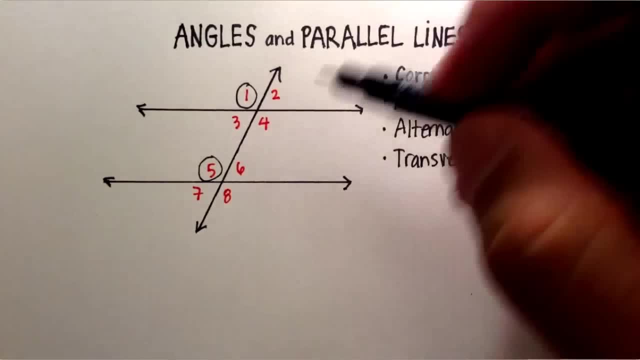 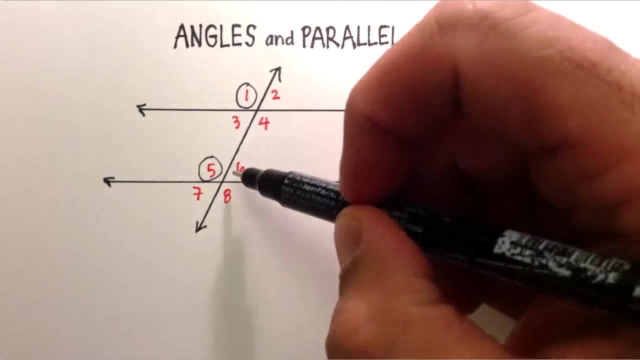 Now let's see if we can name the other corresponding angles in this, in these parallel lines or in this figure. right Now, if you said that two and six are corresponding, you would be correct. I'm just going to draw them a little bit different. 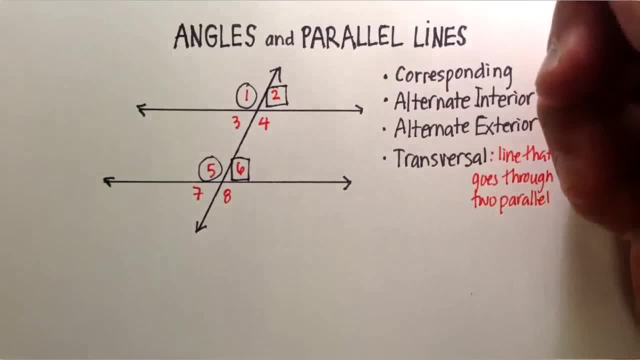 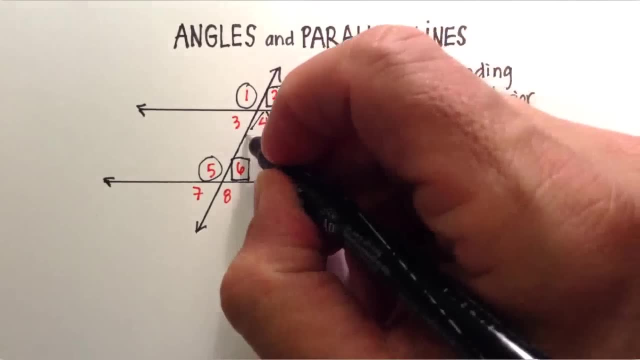 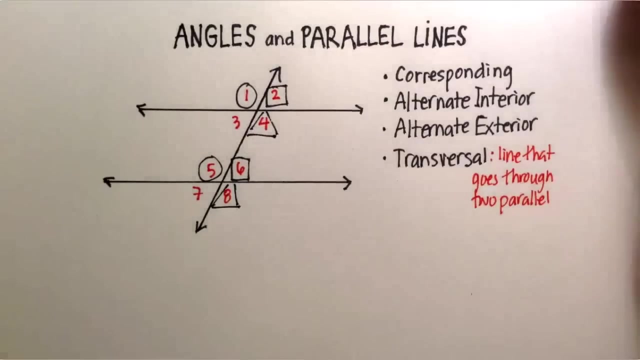 or I'll just put a different figure about them, so we know that they're corresponding, right? If you said that four and eight are corresponding again, you would be correct. Let's just do it that way, Okay. And then, finally, three and seven would be the other corresponding angles. 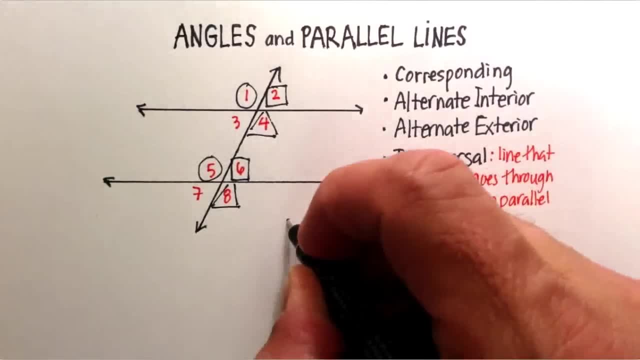 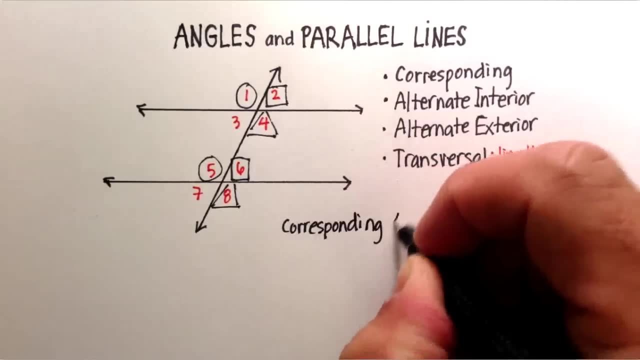 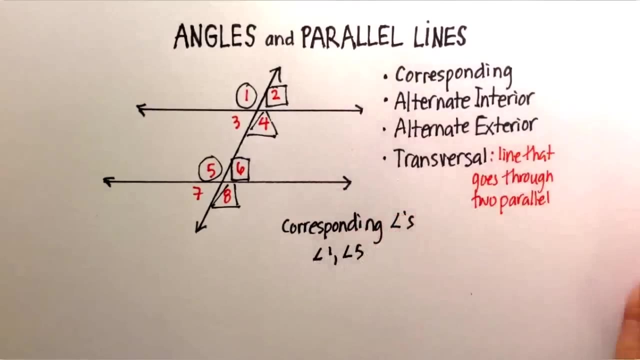 And you can just do it like this, You know, we'll just say: here's corresponding, We'll just call this a category: Angles- remember that's the symbol for angles- And we'll say that angle one, angle five are corresponding. 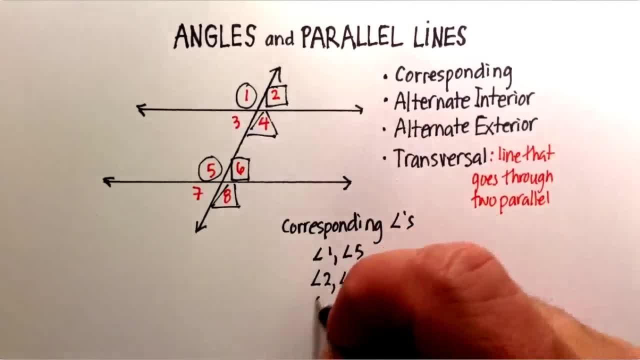 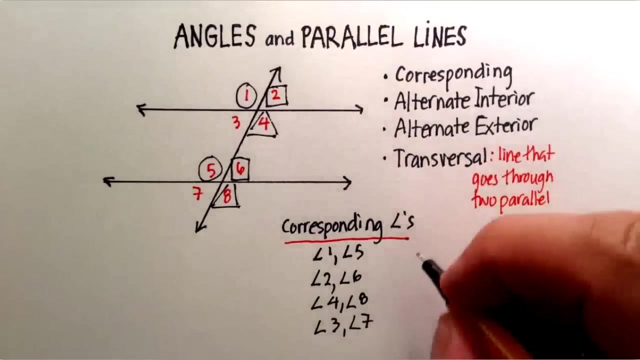 angle two, angle six, angle four, angle eight, and angle three, angle seven. Okay, These would be our corresponding angles. Now, the thing about the corresponding angles through parallel lines is that they're all equal or they're all congruent. 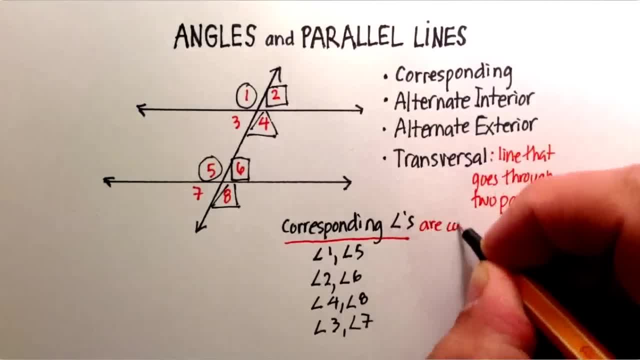 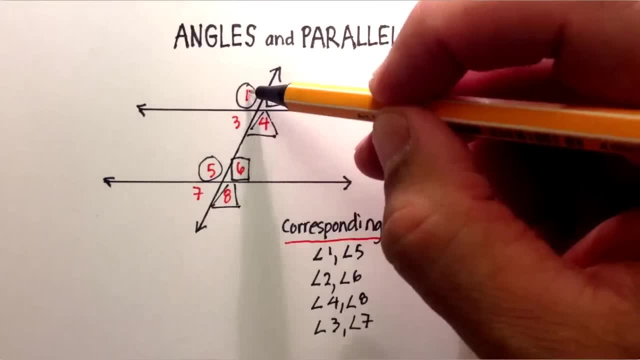 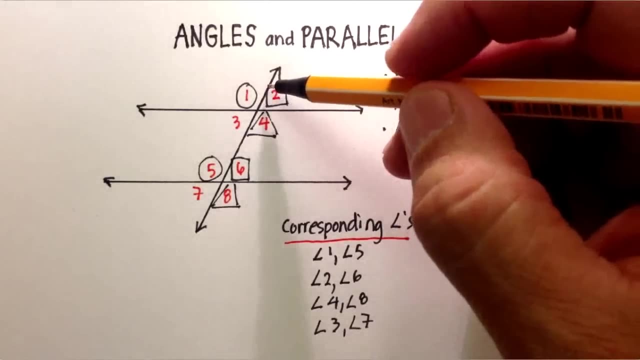 So corresponding angles are congruent. Okay, so if you look at that, you'll see that, for example, angle one and angle five- they're both obtuse angles, right? And if we took our protractor and measured these, we'd see that they're both the exact same number of degrees. 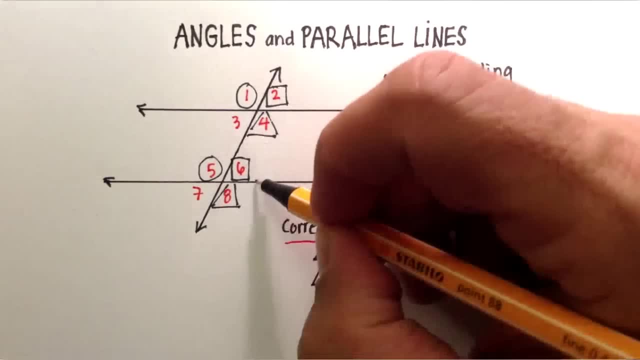 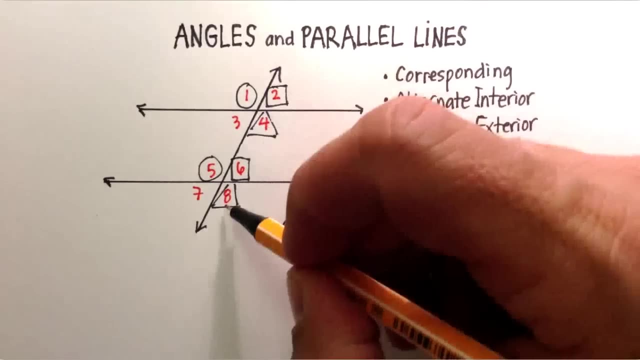 You'll notice that two and six are both acute angles and again they would be corresponding and therefore they are also congruent with parallel lines. You can see the same with four and eight. Now, what do we know about four and eight? 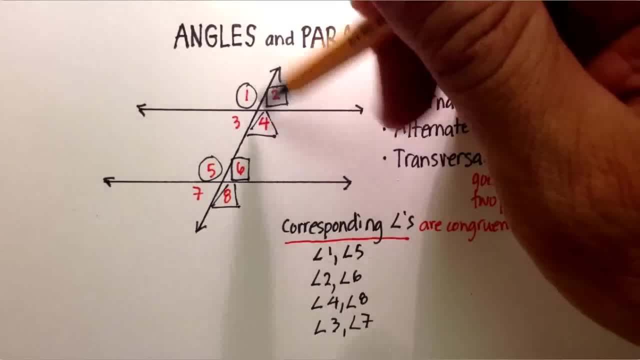 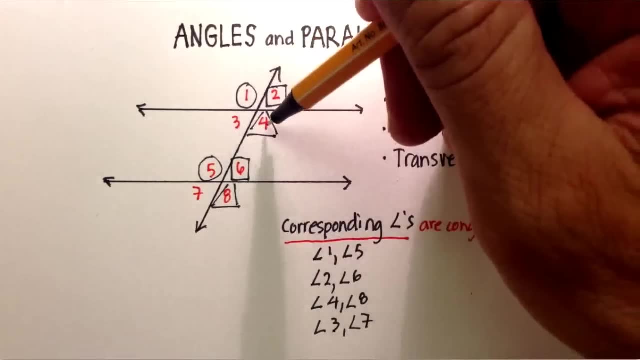 Well, they also form vertical angles, don't they? Which is kind of interesting. So five and eight are vertical angles. So whatever number of degrees one is four is the same. Whatever number of degrees five is eight is the same. 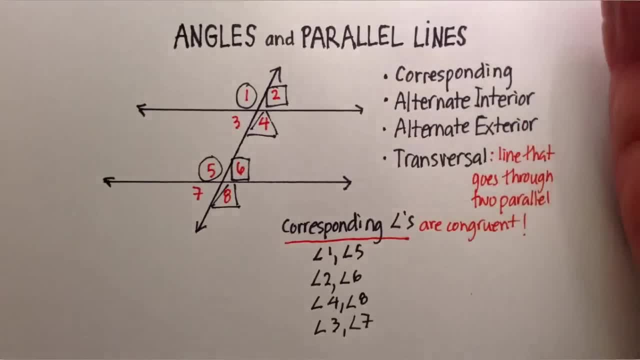 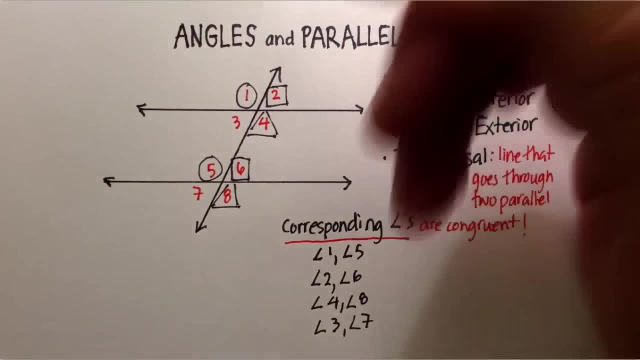 which means that eight and one are also congruent, right, They would be the same number of angles. Four and five would be congruent as well. Three and two corresponding, Seven and six corresponding. They're the same number of degrees. 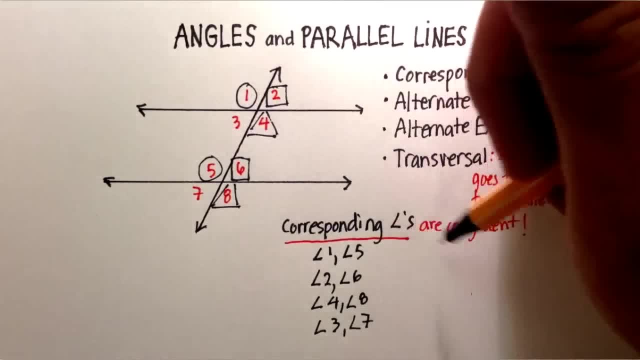 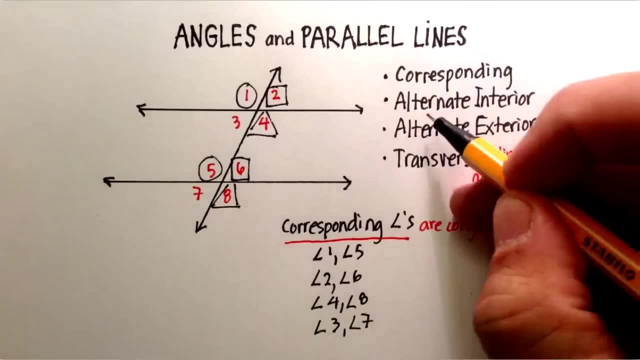 So all sorts of interesting relationships start to happen here with corresponding angles through parallel lines, And that's kind of the introduction that I wanted to talk about when we talked about alternate interior angles. Okay, so let's go ahead and write that out as a category. 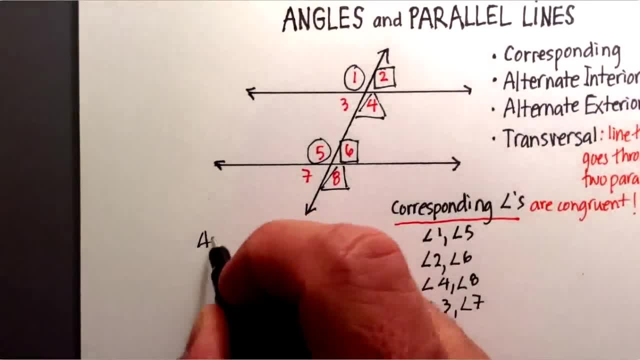 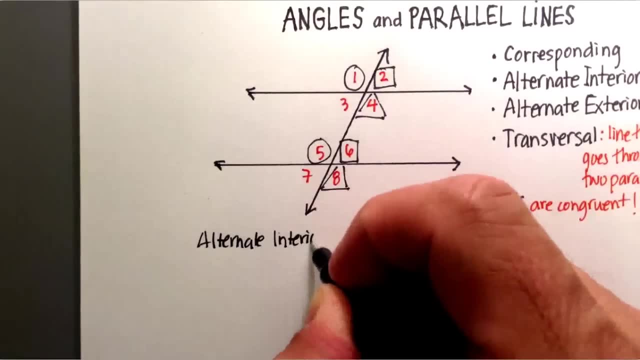 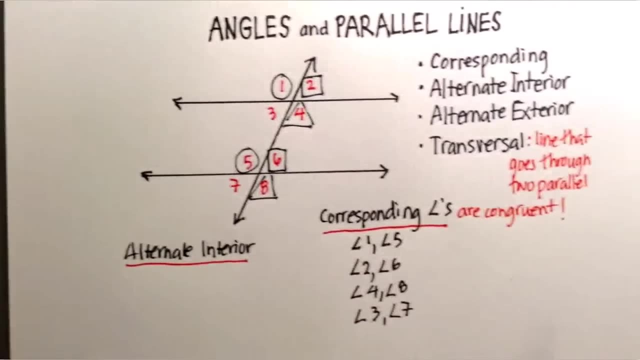 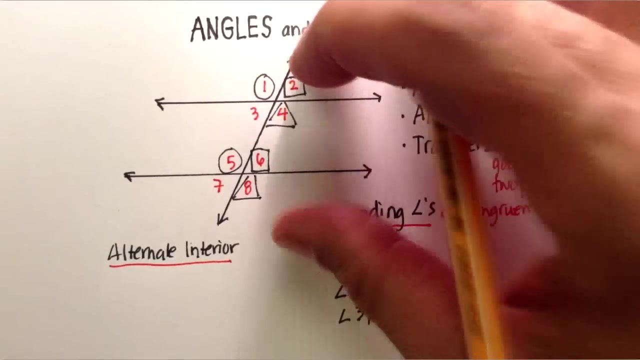 Let's move this over to here. Alternate interior angles. Now let's think about what interior means. If you were to look at this, you would see that these would be three, four, five and six are between the two parallel lines. 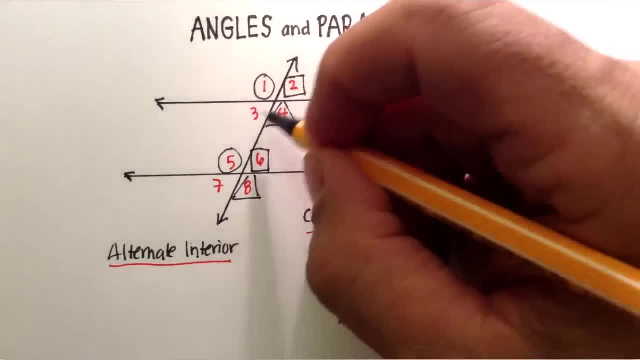 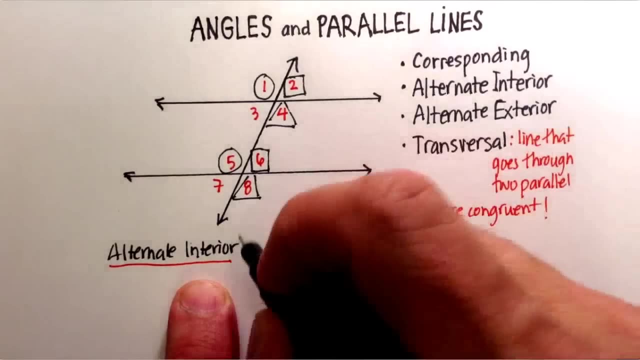 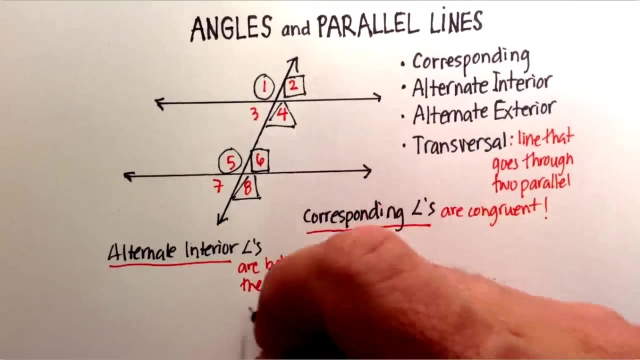 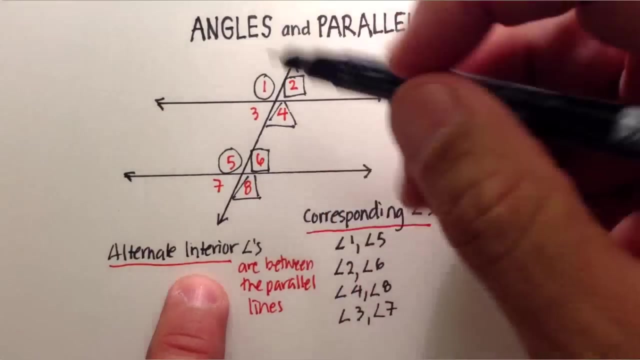 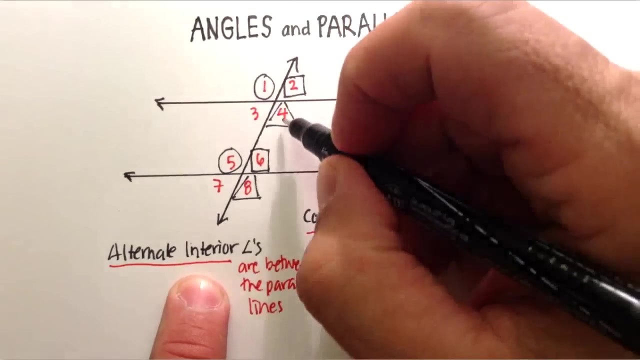 Those would be interior angles. Okay, because again, they're in between the two parallel lines. So alternate interior angles are between the parallel lines, Are between the parallel lines, And here's what's interesting about the alternate interior. Now remember what we said about one and four being vertical angles. 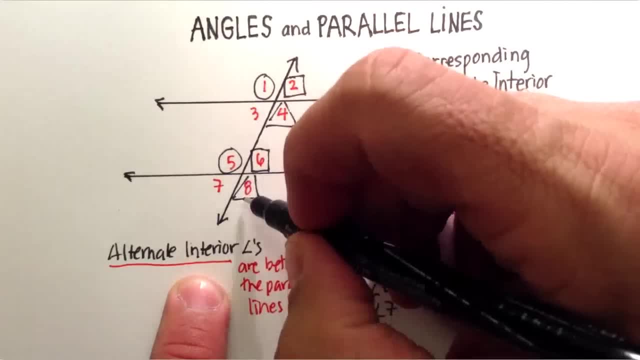 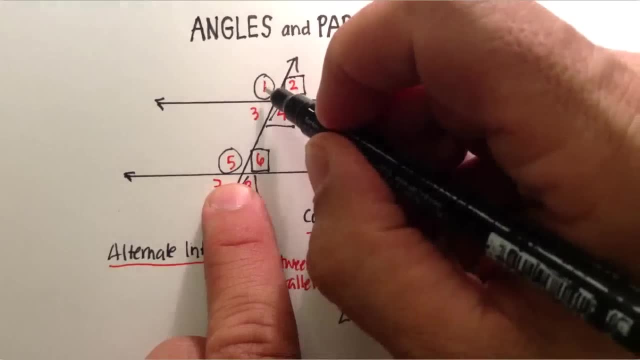 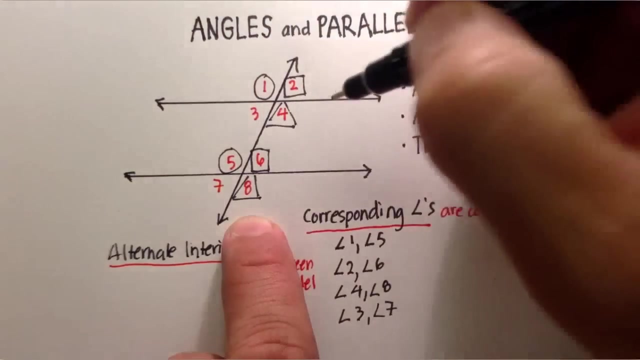 five and six being vertical, five and eight rather being vertical angles. Since we know that one and five are congruent and we know that one and four are vertical and five and eight are vertical, that must mean that the four and the five are congruent. 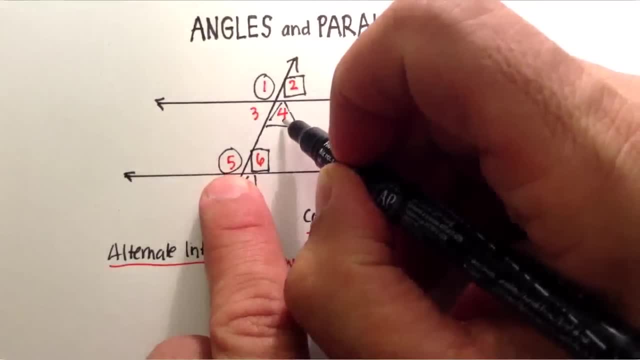 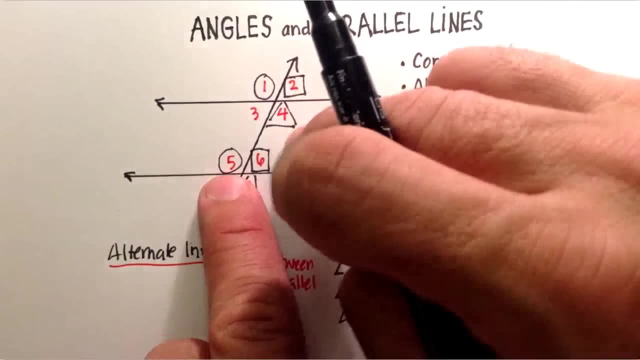 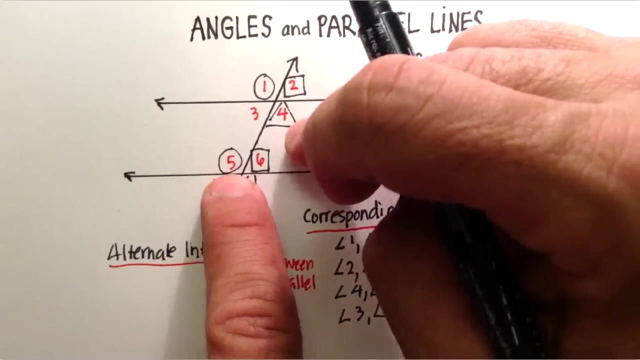 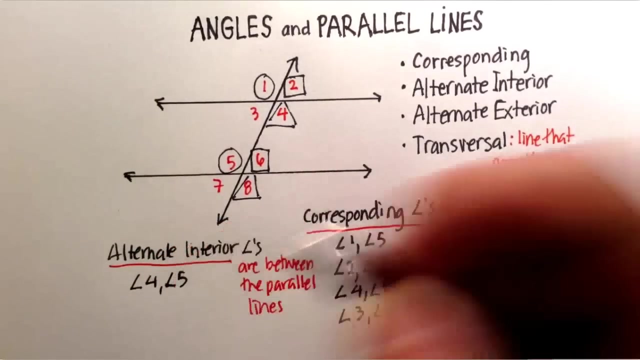 Four and the five are congruent And notice that they're on alternate sides of the transversal And that's why we call them alternate interior angles. So four and five are alternate interior angles And they're congruent. So not only corresponding angles are congruent. 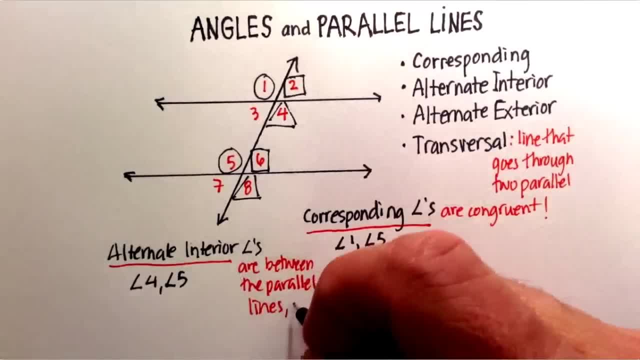 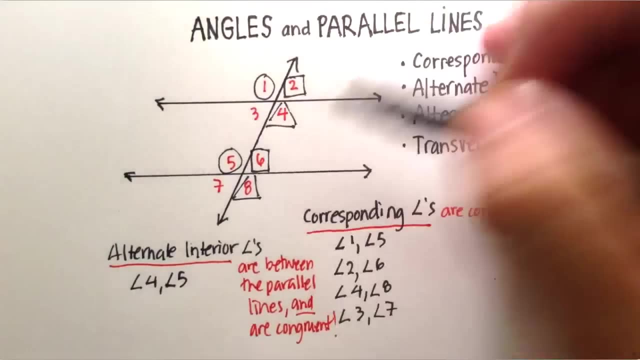 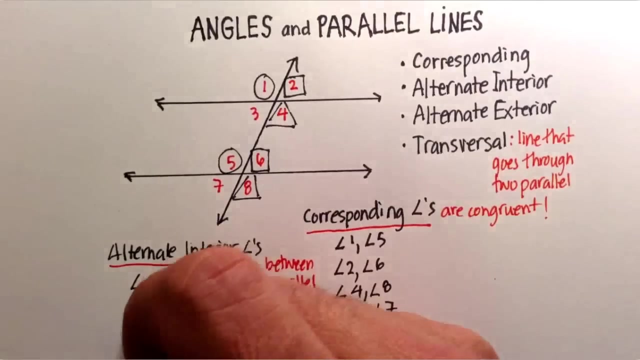 but alternate interior angles are between the parallel lines and are congruent. Can you name any other alternate interior angles here? We said four and five are. If you said three and six again, you'd be correct. And why are they alternate interior? 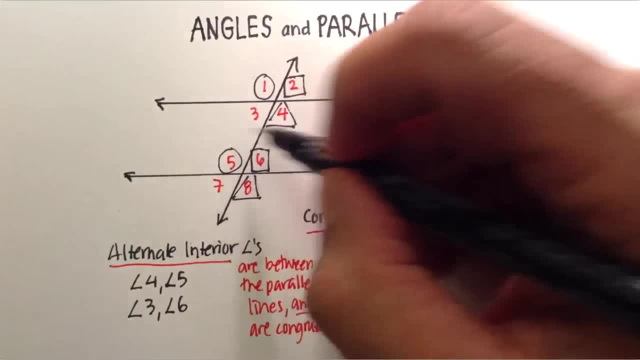 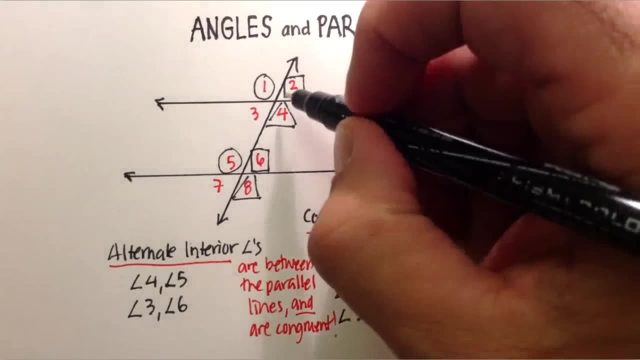 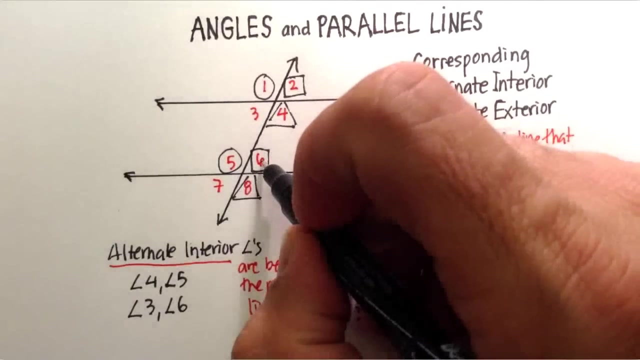 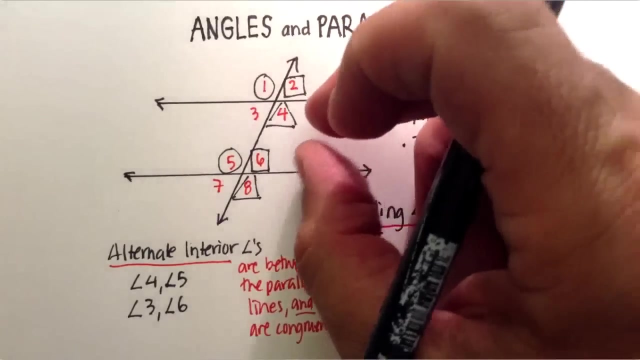 Well, the word alternate again. the word alternate means that they're on alternate sides, opposite sides of the transversal line, and they're also congruent because three and two are vertical, seven and six are vertical and two and six, and three and seven are corresponding. 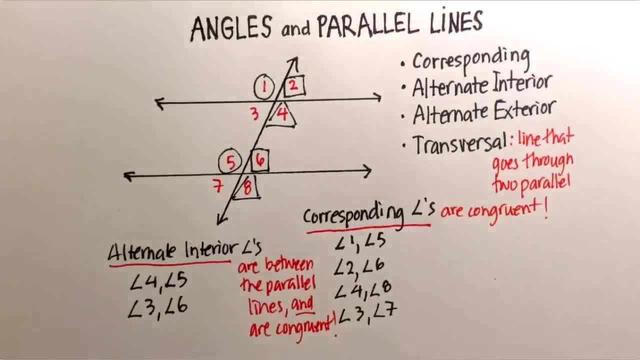 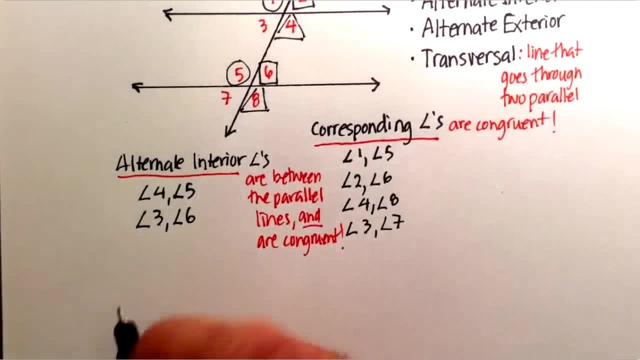 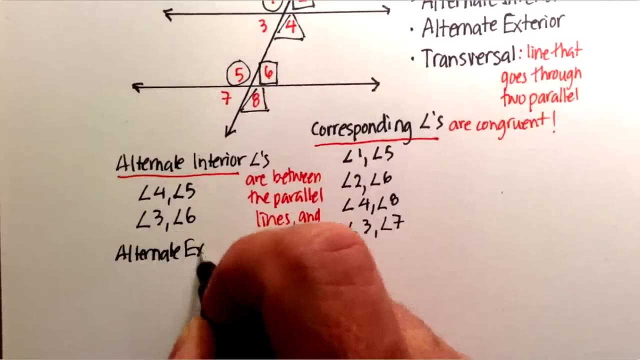 So these are also congruent. You can probably guess what's going to happen with the alternate interior angles, So let's just go ahead and write a new category down here: Alternate into exterior. excuse me, Now again, let's see what the words mean. 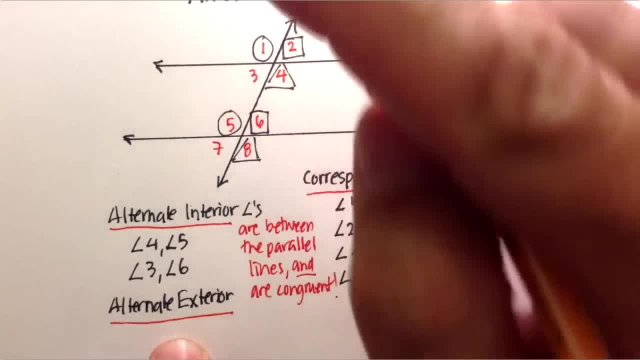 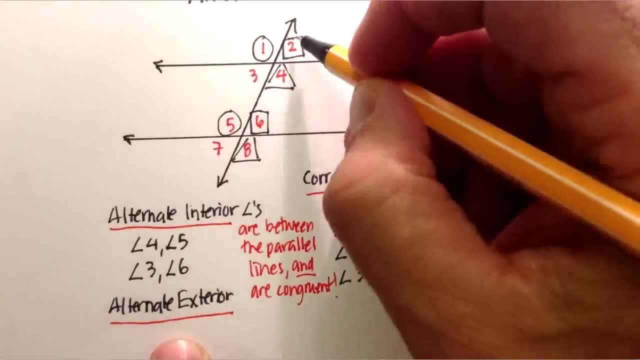 Alternate again means on opposite sides Of the transversal. now okay, So one, three, five and seven are on the alternate side of two, four, six and eight. We know that And we're looking at the exterior angle. 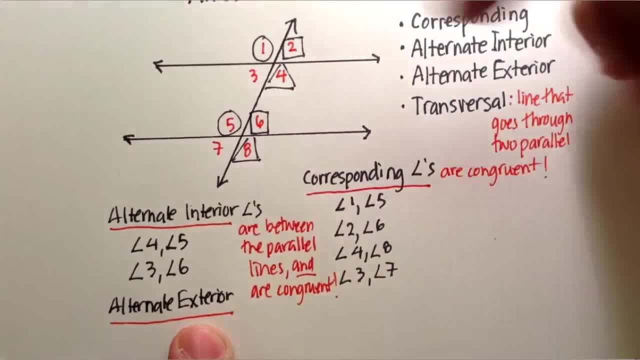 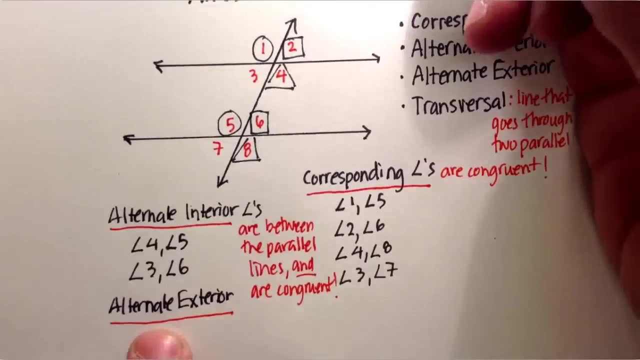 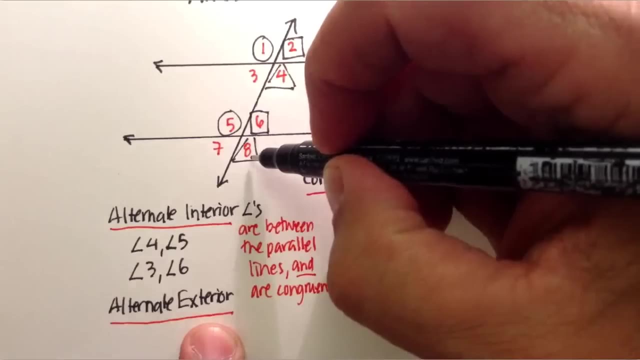 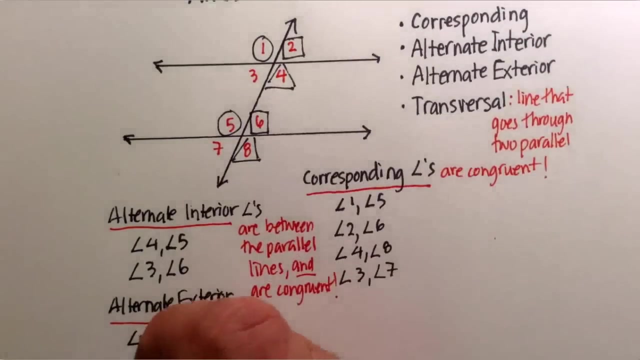 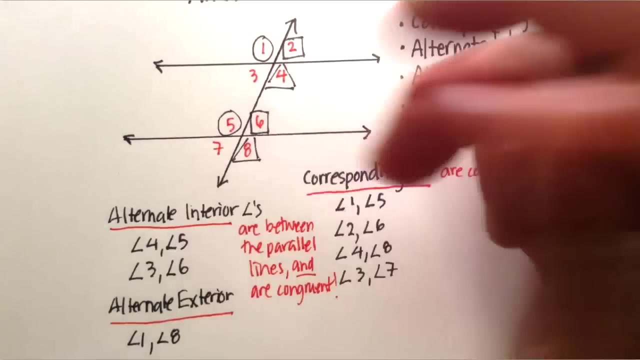 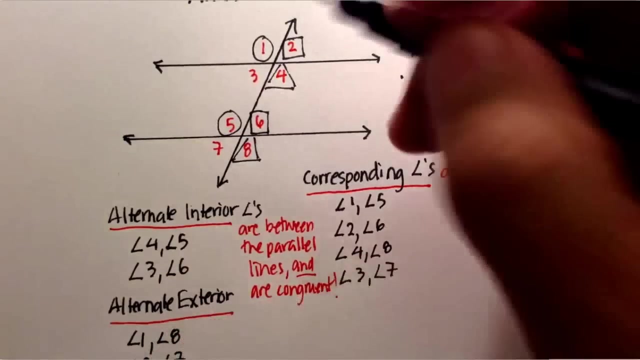 So if we eliminate the interior, the exterior would be one and two, seven and eight. So let's see what alternate exterior means. One and eight would be alternate exterior angles. okay, Two and seven are alternate exterior angles And again they would be congruent. 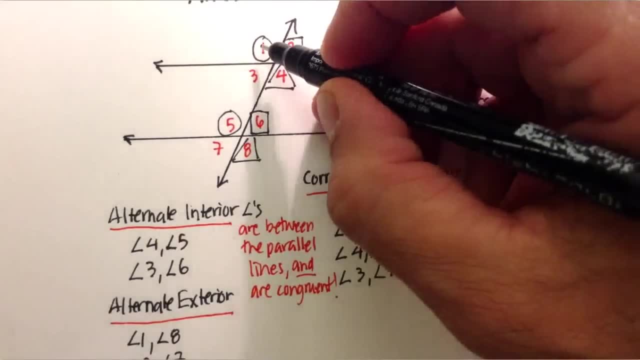 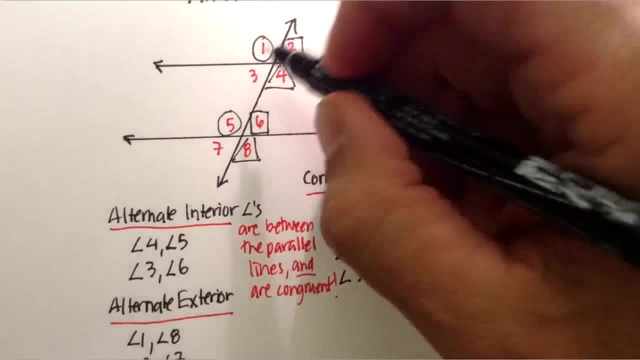 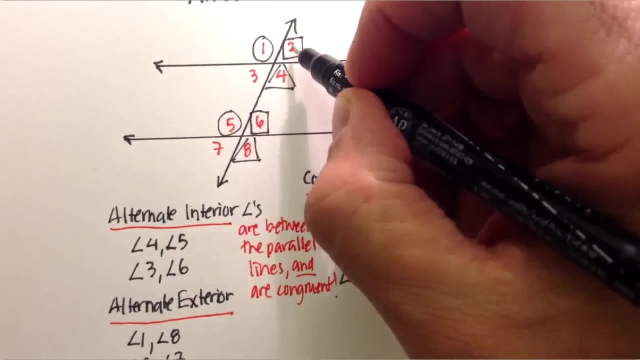 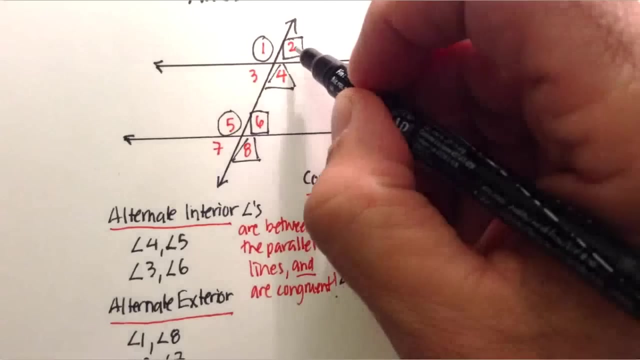 for the same reasons that we talked about right. One is congruent with four. Four is corresponding with eight, So one and eight would be congruent. Two is corresponding with six. Six is vertical to seven. That means that two and seven are alternate exterior angles. 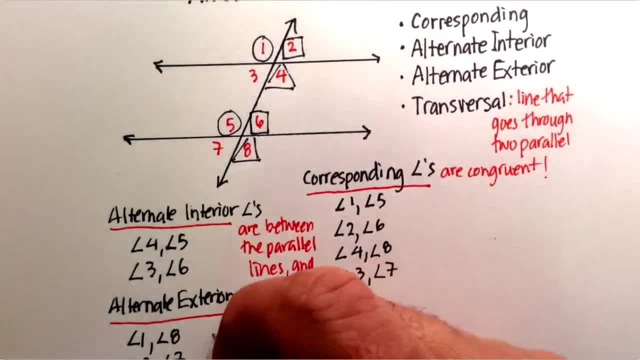 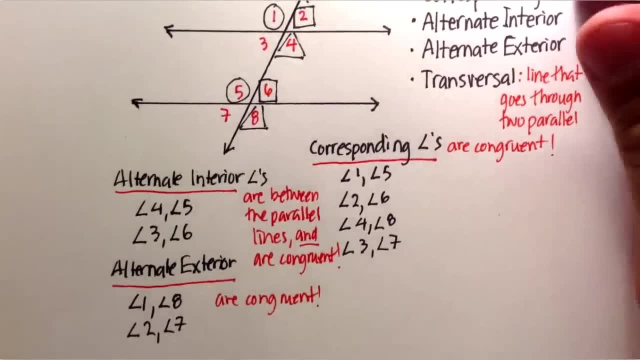 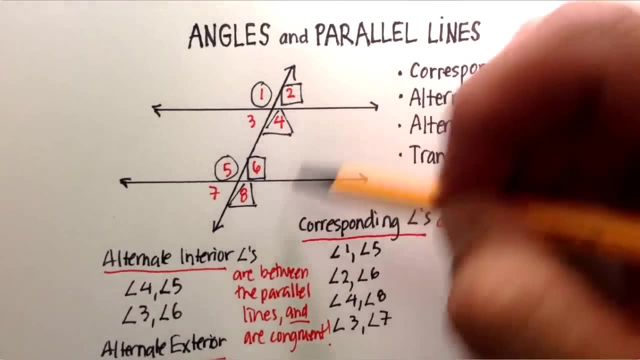 and they are also congruent. Okay, so I hope this was helpful. Again, the transversal that cuts through parallel lines creates all sorts of interesting relationships with the angles that they're formed. okay, And again, just look at the word corresponding. 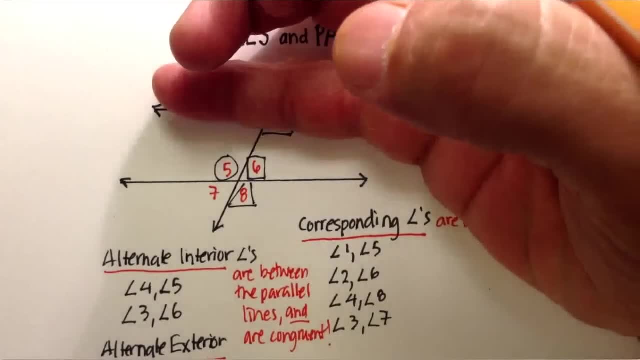 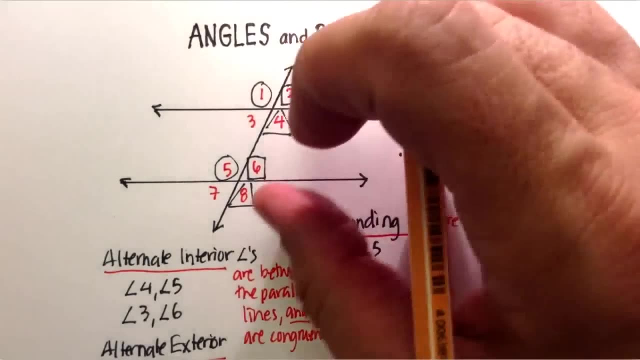 Just think of these as two little separate groupings of four and just think of that. they're in the upper left, upper right, lower right, lower left, In the same spots, right, Alternate interior. just think of the lines or the angles in between the two parallel.